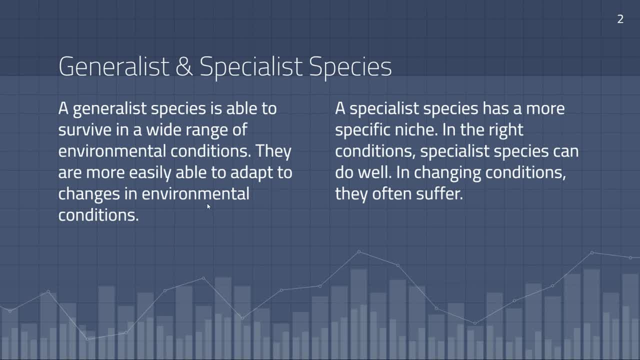 Just a reminder that a generalist species is a species that's able to survive in a wide range of environmental conditions. So remember there are lots of different environmental conditions that can affect individuals within a population. For example, the temperature, the pH. These are different conditions that can have an effect on a species. 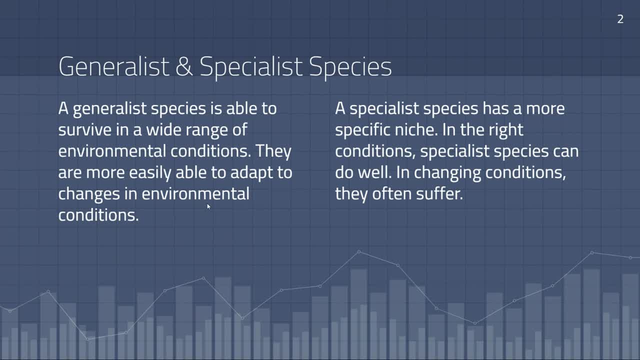 And so generalist species are typically more easily able to adapt to changes in those environmental conditions. A specialist species, on the other hand, has a more specific need, And so what that means is that, in the right conditions, we can see populations in those specialist species increasing. 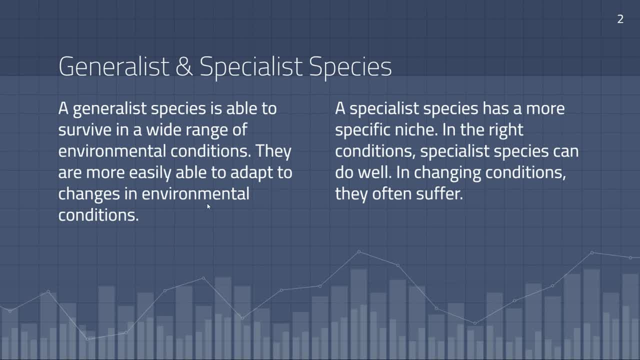 They can do very well, But when those conditions change, if it's not a condition that is very specific to that specialist species, then those species can often suffer, And so a lot of times we see that in the right environment a specialist species will do very well. 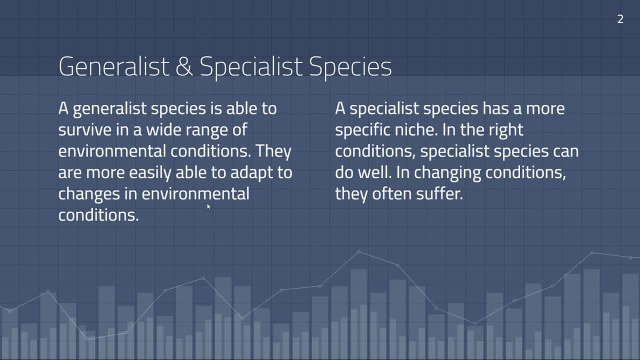 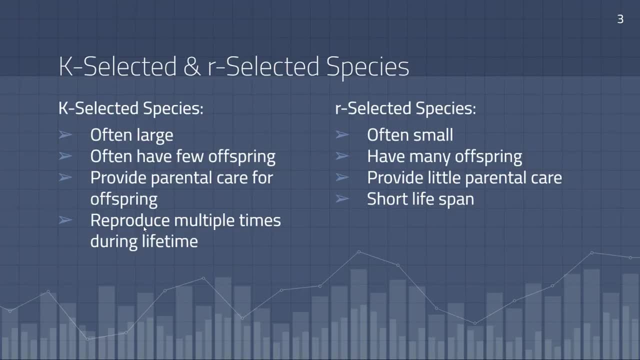 But when that environment changes, that species is no longer able to succeed. We also discussed K-selected and R-selected species, So remember that K-selected species are often large. They are species that have few offspring, So they might reproduce several times during their lifetime. 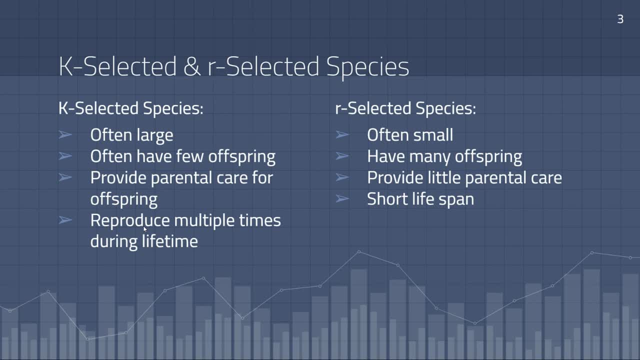 But each time they reproduce, they're typically only having a few offspring each time. However, these species do have a few offspring. However, these species do have a few offspring each time, But these species do provide parental care for their offspring, So they're spending quite a bit of time and energy caring for their young and helping their young learn how to function within the ecosystem. 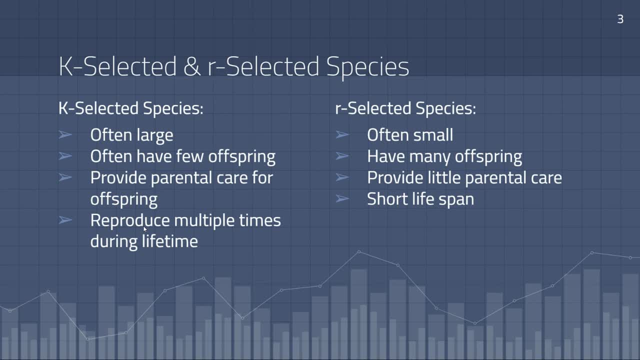 Our selected species, however, are quite different. They are often small, They have many, many offspring, but typically provide very little parental care for their offspring, And quite often they have a short lifespan and die after they reproduce. So they might pass on their genes to the next generation and then that kind of marks the end of their lifespan. 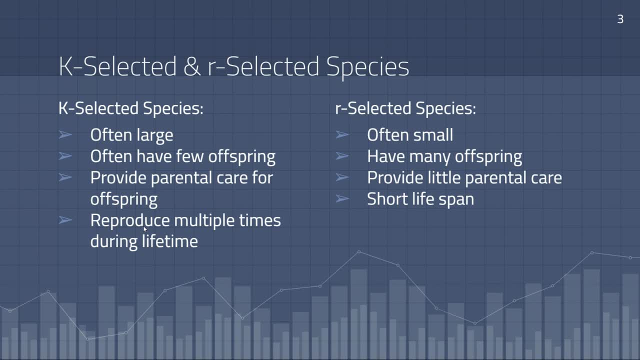 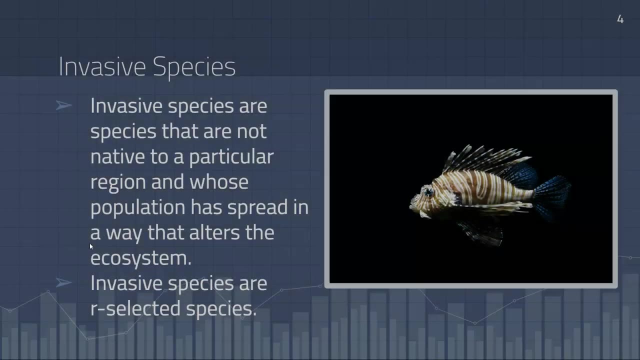 Now in the wild, many species fall somewhere within the spectrum of being a K-selected or R-selected species. Not every species fits clearly into one of these two categories, but instead it can be seen more as a spectrum. You should also be familiar with the term invasive species. 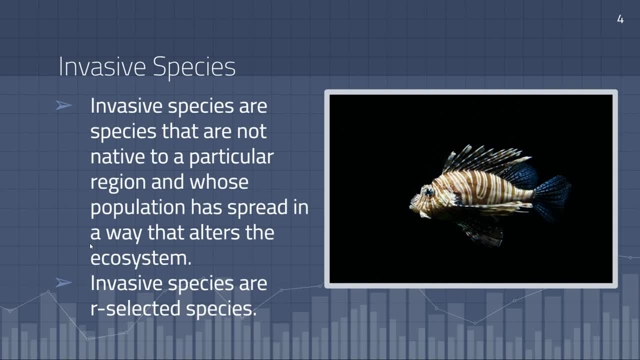 So invasive species are species that are not native to a particular region, yet their population has spread in a way that alters the ecosystem, And so what you can see in the picture here is an example of a lionfish. A lionfish is kind of a notorious invasive species found in the Gulf Coast of Florida. 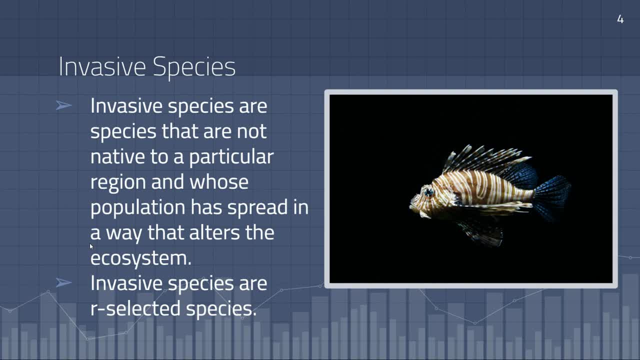 And its population has been increased. It's been able to explode largely due to the fact that it doesn't really have any predators in its ecosystem, And so invasive species are often also R-selected species. Because they are able to produce so many offspring at one time, that can make these species more successful in reproducing and spreading in a way that alters the ecosystem. 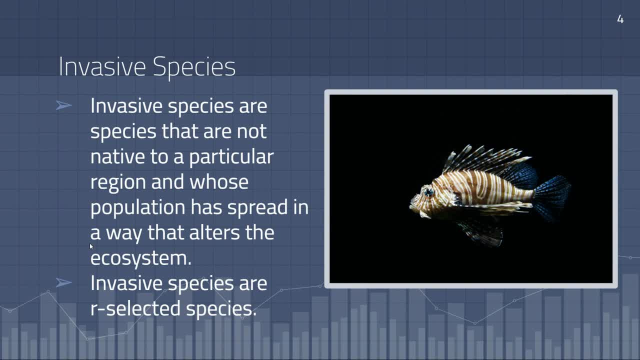 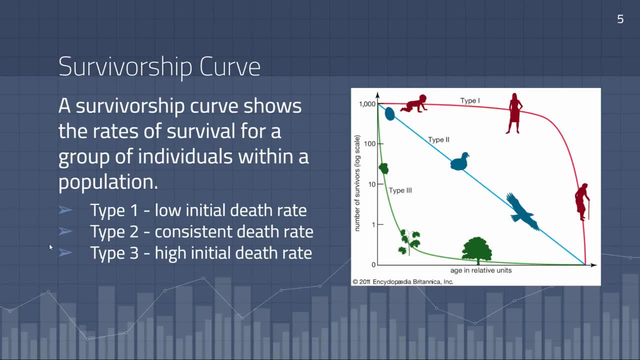 While that might be good for the species, it's typically very, very expensive. It's very bad for the native plants and animals in that region, And so we can also represent different species on what we call a survivorship curve, And so there are three types of survivorship curves that you should be familiar with for the AP exam. 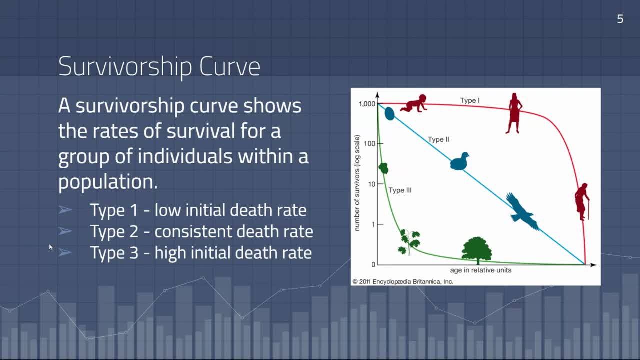 And so the first one we can see here, represented in red, is a type 1 survivorship curve, And a type 1 survivorship curve is a type 1 survivorship curve. survivorship curve, we see organisms that have a low initial death rate. So these are 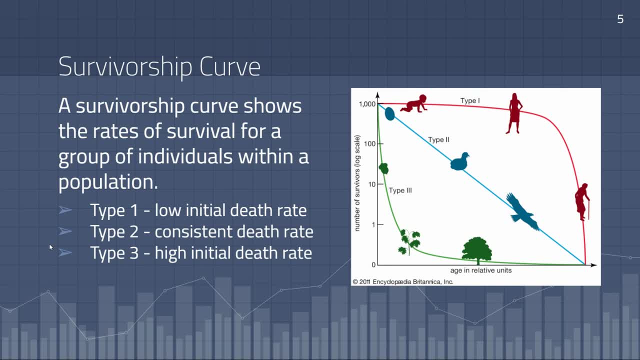 organisms that have a very low initial death rate and in general, many of the organisms survive on to adulthood. So the example you can see in the picture there is a human Humans would be part of a type 1 survivorship curve. Okay, there are many other case-selected species that would also fit. 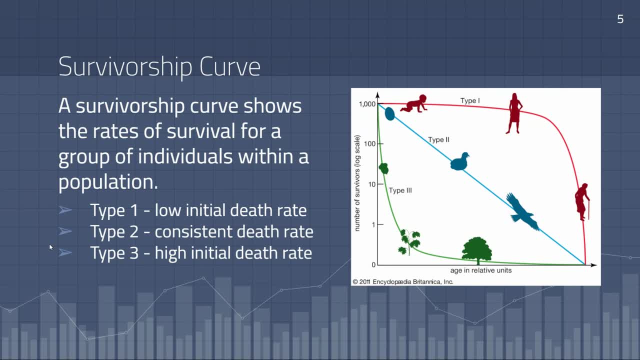 within a type 1 survivorship curve. For example, elephants often live on to adulthood, and so they would be considered a type 1 survivorship species. They have a very low initial death rate. A type 2 survivorship curve shows a consistent death rate through. 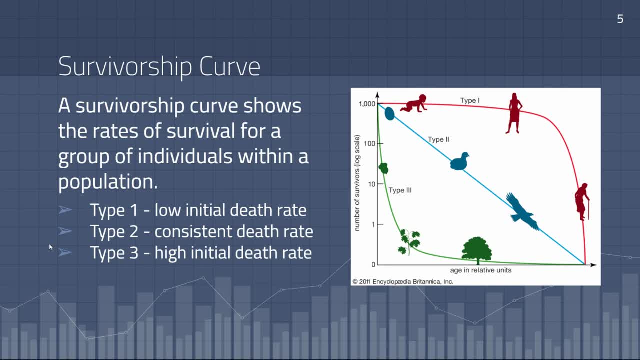 the lifespan of the organism. There are lots of different species of birds, lizards, other small animals that would fit into this curve. It's more of a linear representation here, where we have a very consistent death rate And then finally we have a type 3 survivorship curve. This curve shows a very high 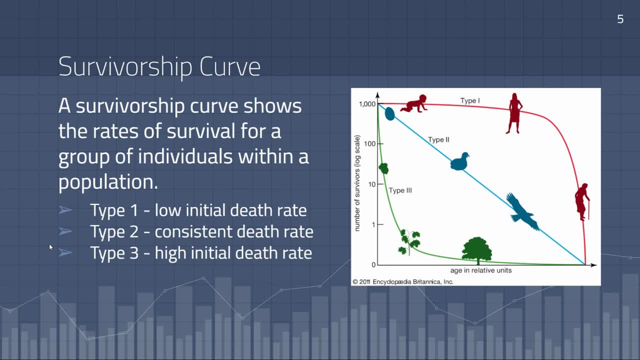 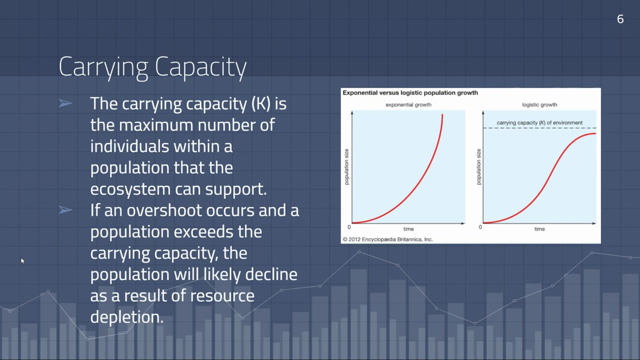 initial death rate. that kind of levels out as the organism moves on in its lifespan, And so we can typically see that a lot of the R selected species fit in to this type 3 survivorship curve, And so whenever we're talking about population in an ecosystem, one thing that's very important to be aware of is 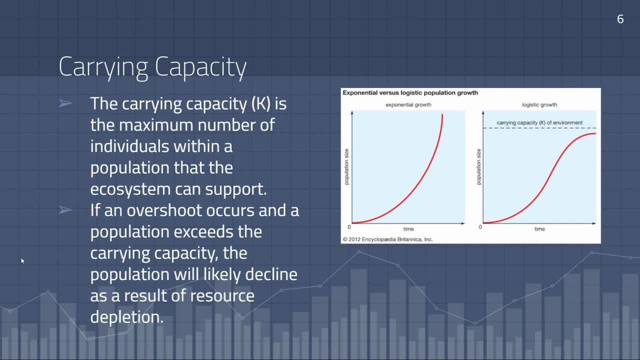 the carrying capacity. The carrying capacity, which you'll sometimes see represented as K, is the maximum number of individuals within a population that the ecosystem can support, And so you can see on the graph here we have exponential growth and logistic growth, And so, you know, a population might continue on showing an. 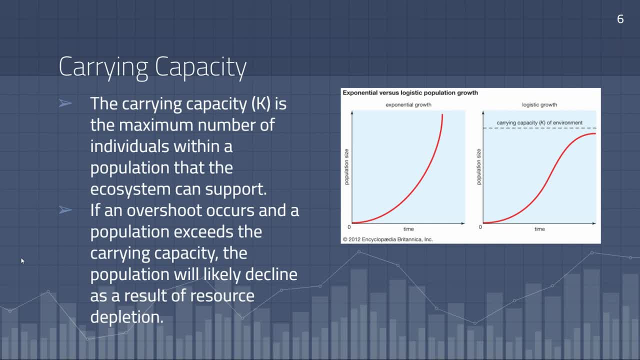 exponential growth curve to a point, but eventually the population will run out of resources, And so that's what we can see here, where this population has kind of hit this point, where it's at the maximum number of individuals that an ecosystem can support. It's the 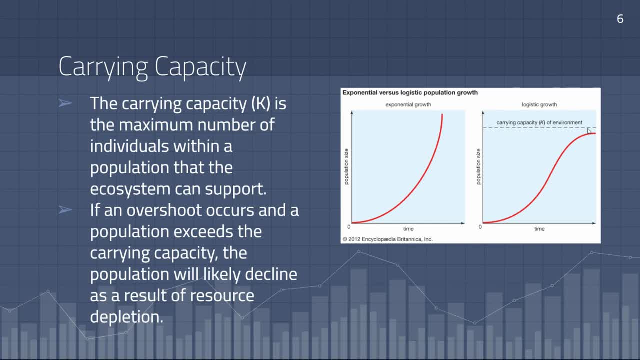 maximum number of food and other resources available if we have more than that number of individuals within the ecosystem And that would show us that an overshoot has occurred. An overshoot occurs when the population exceeds the carrying capacity And, as a result, the population will typically decline. 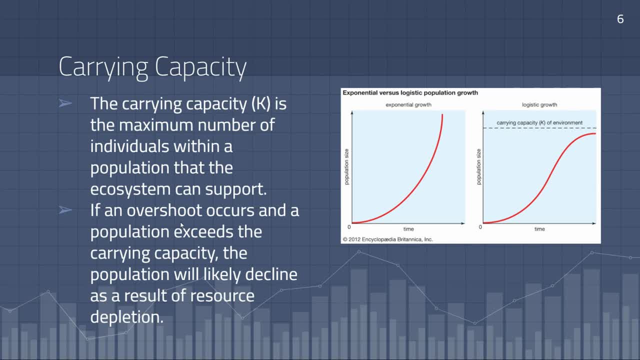 to decrease. This fluctuates the story, so we also know that, as a result, the population will typically decline, because the longer So an overshoot occurs when the population exceeds the carrying capacity And, as a result, the population will typically decline, considering because those resources have been depleted. 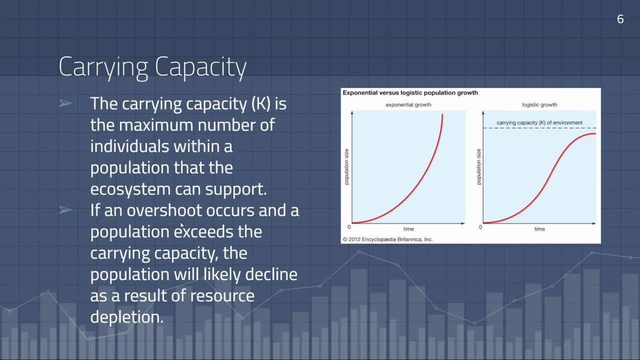 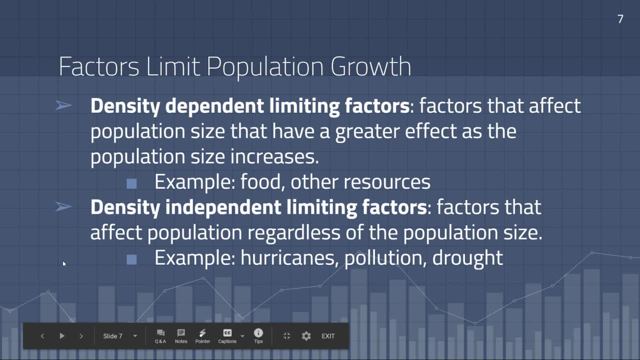 So carrying capacity goes hand in hand with the amount of resources that are available in a particular area, And there are some other limiting factors that we should be aware of, So you need to be familiar with this term. density-dependent limiting factors. Density-dependent limiting factors. 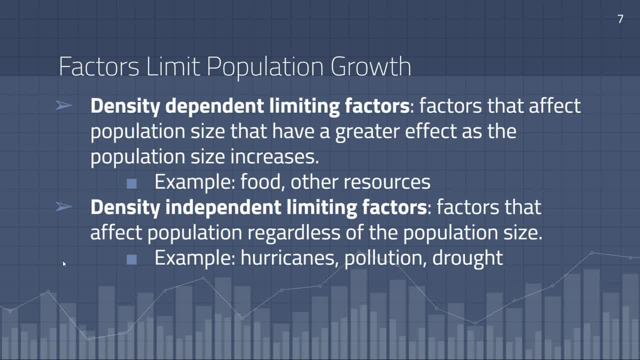 are factors that affect population size that have a greater effect as the population size increases. For example, food is a density-dependent limiting factor because as the population gets larger, the pressure on the amount of food available also continues to increase. If there are more individuals, there's less food available. 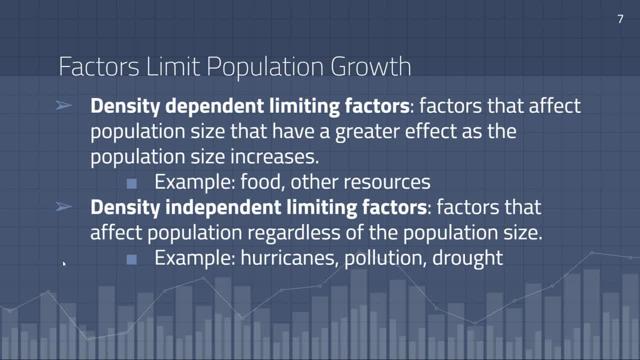 And so food and population size go hand in hand. they're directly related. A density-independent limiting factor is a factor that affects population regardless of the population size. So this is independent of the density of the population. So it does not matter how many individuals 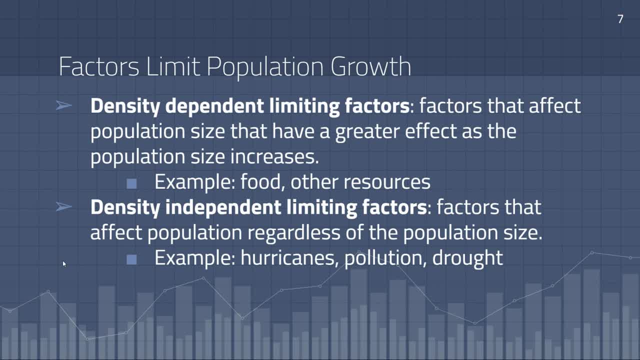 you have in an area, these factors will still have an impact on the population. For example, hurricanes or other big storms. It can have an impact on a population and it doesn't matter how many individuals there are. it can still have a massive impact. 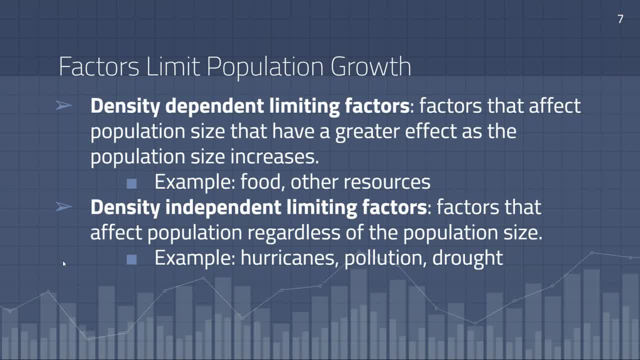 Pollution, especially in a waterway or something like that, could impact an ecosystem, and it doesn't matter how many individuals there are. it can still impact that ecosystem in the same way. Drought would be another example. So as we have a drought, we might. 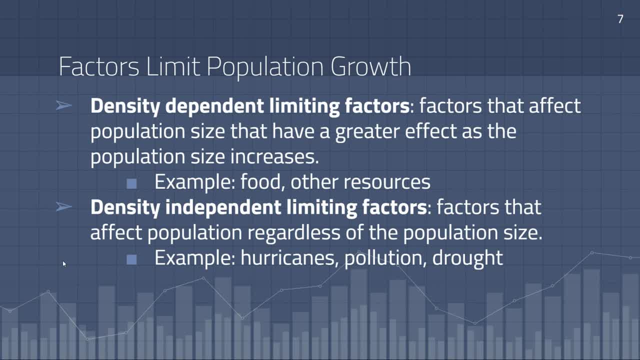 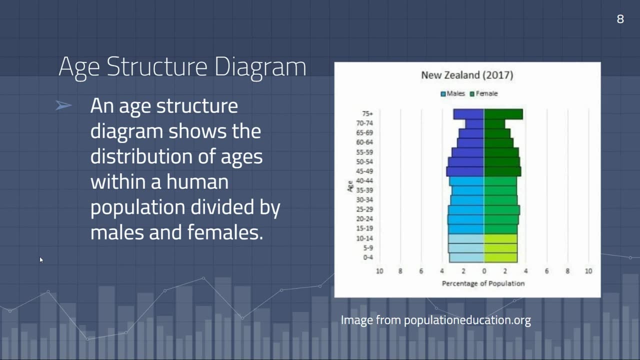 we might have a ripple effect of other consequences that go through the ecosystem, And so these limiting factors that we've discussed also relate very closely to human populations and how human populations can be impacted and changed over time, And so one of the things we talked about 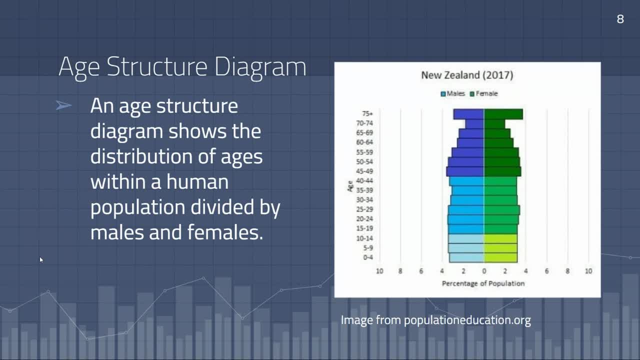 specifically related to human populations were these age structure diagrams, And we discussed how an age structure diagram shows the distribution of ages within a human population divided by males and females. So males are represented on one side of the diagram and females are represented on the other. 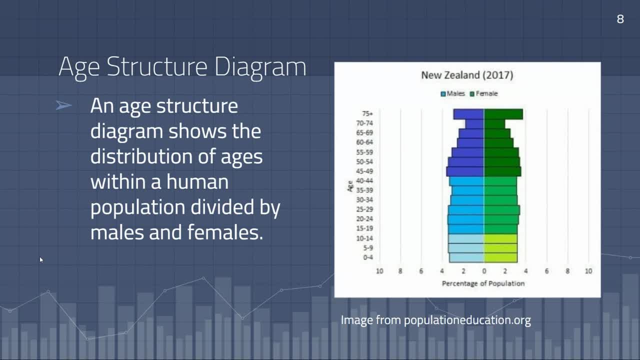 And so an age structure diagram can be constructed for any country, and we can use this to draw some conclusions about the population growth within that country. When we see that the proportions of individuals in each category are relatively equal, that shows us that the population is fairly stable. 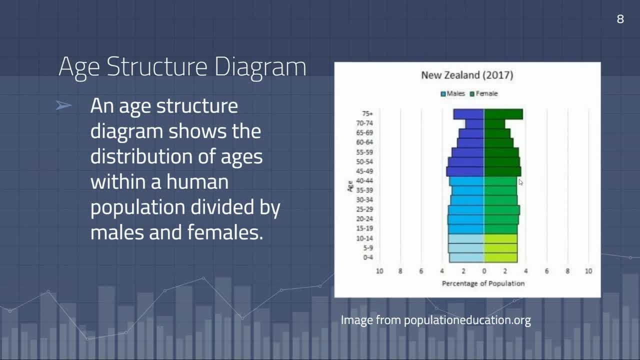 So what we can see here with New Zealand is that this population is fairly stable. They're not experiencing massive population growth. On the other hand, if we saw more of a triangle shape, where we have a very large proportion of individuals in these lower age groups, 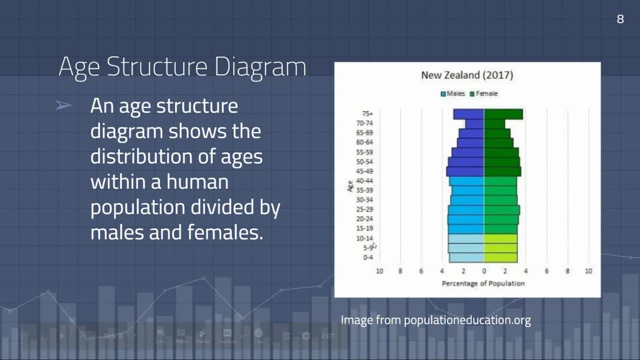 in their pre-reproductive and reproductive years. that would show us the population is likely growing. When we have a large proportion of individuals that are in those younger categories, when they produce kids in the future, they will continue to cause an increase in the population growth. 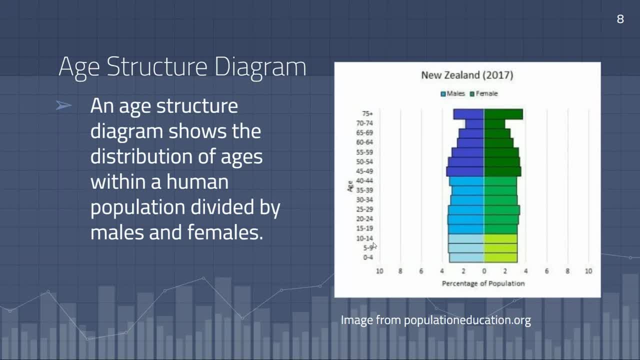 On the flip side. if we have kind of an upside down triangle shape where we have a very large proportion of older individuals in a much smaller group or a much smaller proportion of younger individuals, that typically shows us a decline in population. This kind of age structure diagram is not as common. 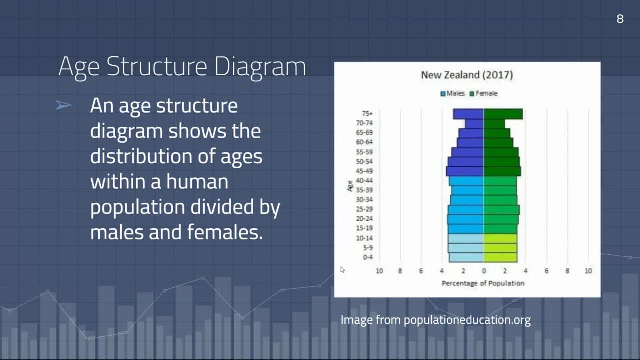 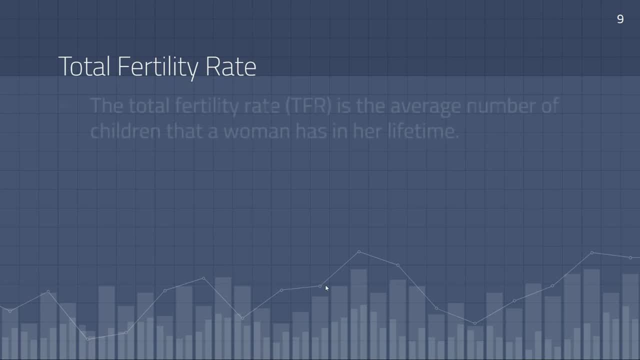 but can be seen in a few countries. Another term we discussed that you need to be familiar with is the total fertility rate. The total fertility rate, abbreviated TFR, is the average number of children that a woman has in her lifetime, And so we typically find that countries. 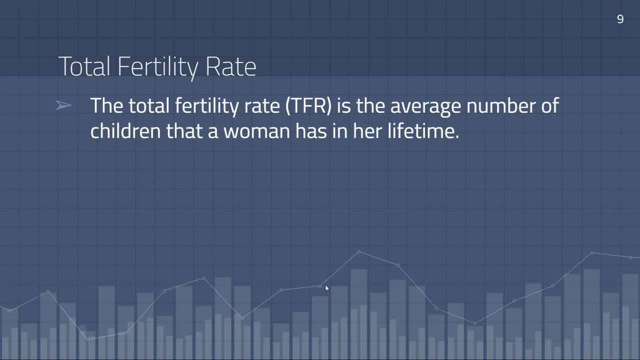 that have a larger population growth also have a higher total fertility rate. Several different factors can impact the total fertility rate in a region, For example, the average age at which women have their first child, If women start having children at a younger age. 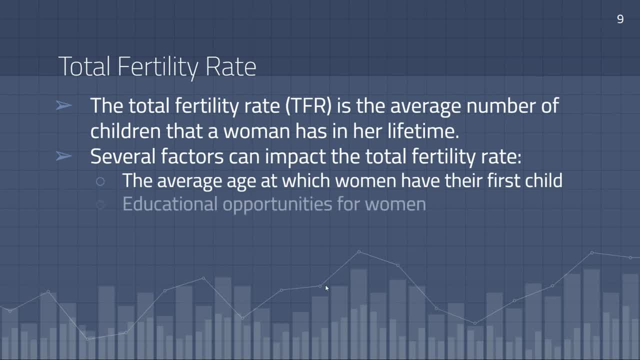 they typically do have more children in their lifetime. An example of this is educational opportunities for women. If women have lots of opportunities to further their education and to start careers, they tend to delay having children and may not have as many children Access to family planning. 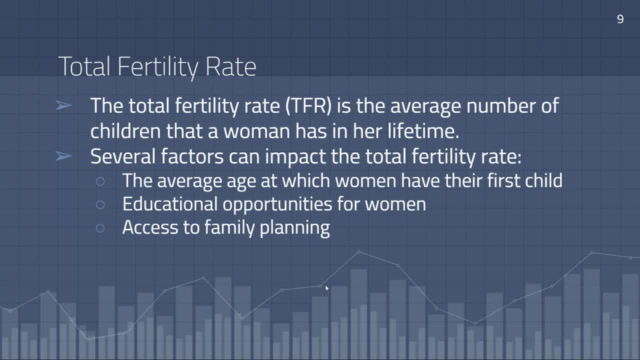 So in some developed countries, families have access to birth control and other methods to limit their family size. In many developing countries, this is not an option, And so a good example of this is a group of women, a single mom, If you're in your third or fourth year in the United Kingdom. 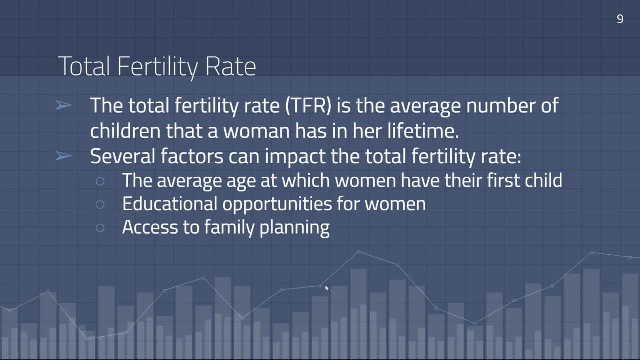 That can also impact the total fertility rate in an area. Government policy can have an impact on the total fertility rate. In places like China, with the one-child policy, the population size of the family was limited due to that government policy. One other thing to be aware of here is that women access to health care can influence infant mortality rates. 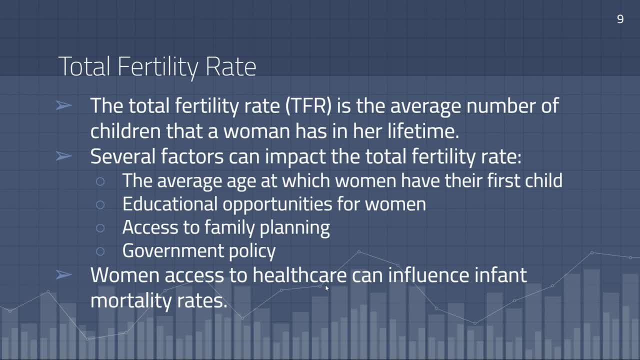 And so, right along with educational opportunities for women, opportunities for health care can have a big impact on the family as well, And so when women have access to health care facilities, they are more likely to be healthy, and their children are more likely to be healthy. 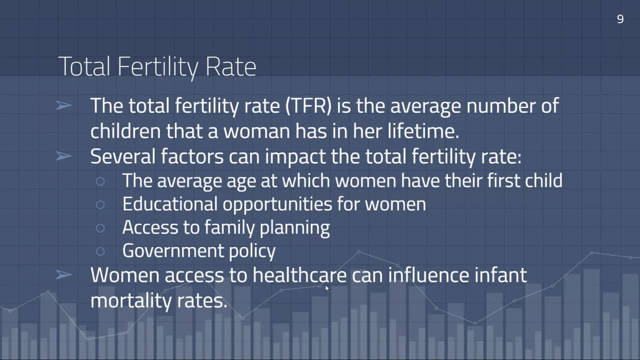 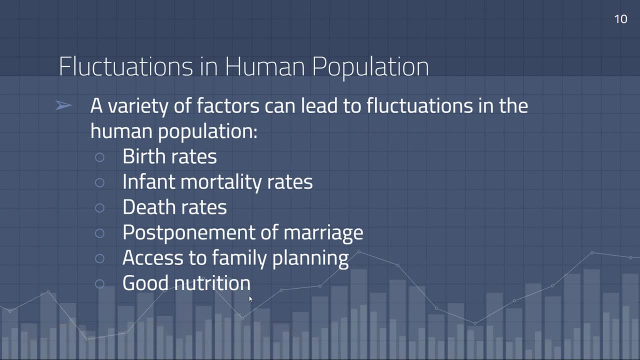 Women who do not have access to these sort of facilities often are living in countries that have a higher infant mortality rate, And so there are lots of different factors that all together can lead to fluctuations in the human population. Obviously, we have discussed birth rates. 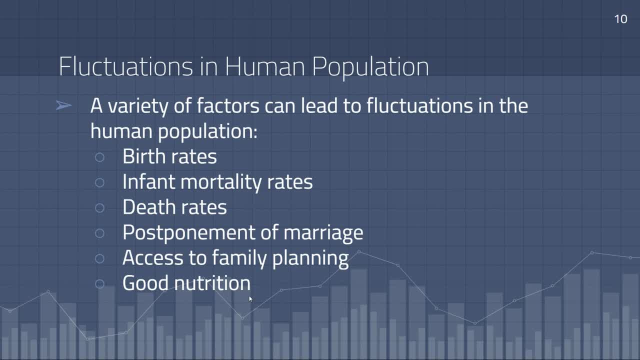 If we have a high total fertility rate in an area we likely have a growing population, Infant mortality rates can also play a role in that, And so if there's a high infant mortality rate, that overall can lead to a rise in infant mortality. 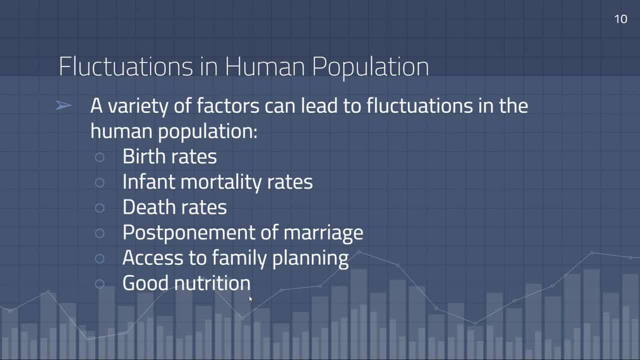 And so that can lead to a rise in infant mortality. And so if there's a high infant mortality rate that overall can lead to a rise in infant mortality, to a slight decline of that population. Death rates can have an impact Typically more developed. 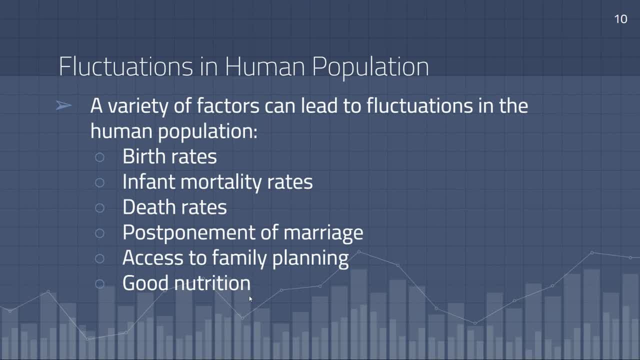 countries have greater access to health care than those developing countries, and so, in general, people may live longer lifespans in those more developed countries. Postponement of marriage can have an impact on human population because that goes right hand in hand with birth rates, because women who delay marriage typically have kids later in life or may not have as many kids. 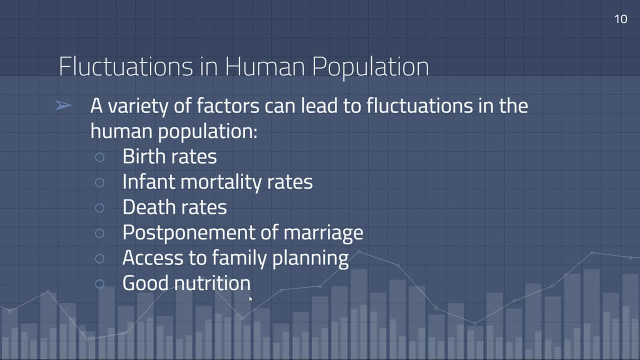 whereas those who get married earlier- especially in some countries where women are expected to get married very young- typically have more children. Access to family planning can also have an impact on human population, and so some individuals in developing countries that don't have access to any form of 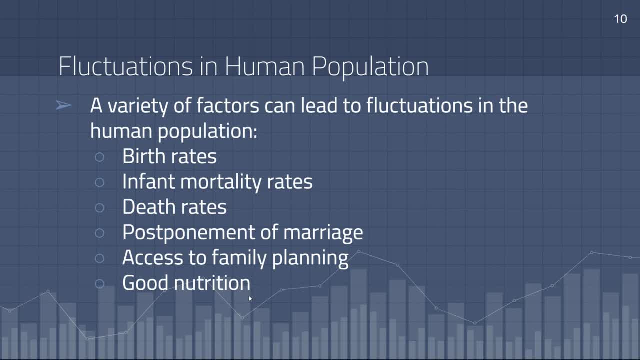 education related to family planning typically have larger family sizes. And then, finally, nutrition can have a big impact on human population. So the availability of nutritional foods in an area can impact the population. in certain areas where good nutritional food is not available or where food is more scarce, The lack of food and malnutrition can have a negative impact on. 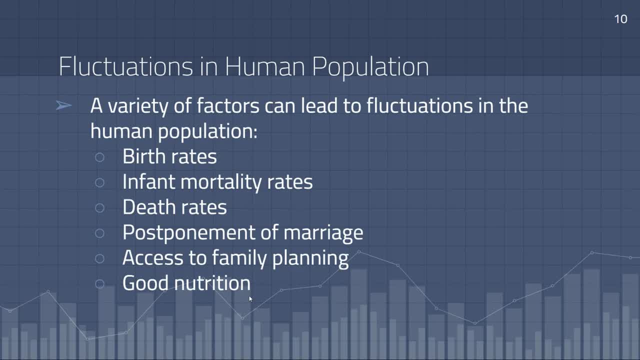 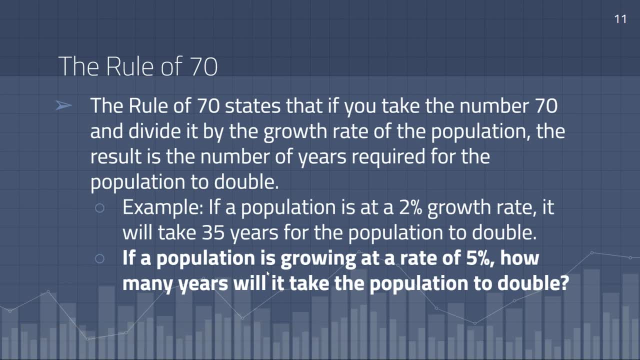 impact on the human population, And so one other thing that you need to be aware of when it comes to human population and the study of human population is the rule of 70. So you need to practice the math on these sorts of questions. The rule of 70 states that if you take the number 70, 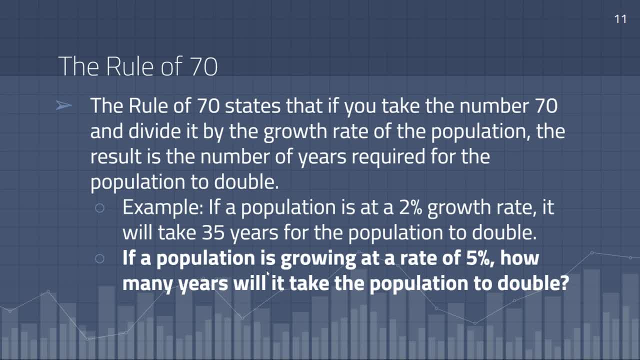 and divide it by the growth rate of the population. the result is the number of years required for the population to double. So if a population is at a 2% growth rate, it will take 35 years for the population to double. So I took 70,, divided it by that 2% growth rate and I got that 35 years for the population. 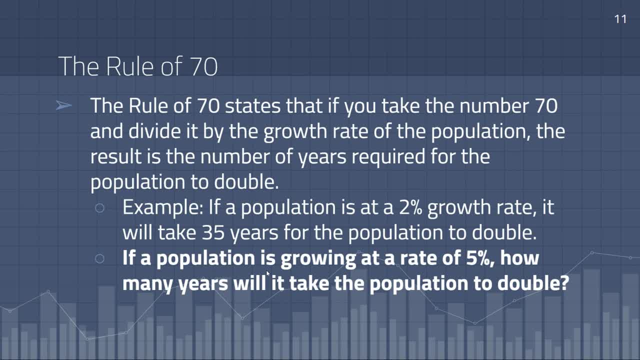 to double. So even though 2% may not be the number of years required for the population to double, it may seem like a very modest growth rate, When we're looking at a massive population, even a 2% growth rate can really be a tremendous growth rate over time. So in just 35 years, 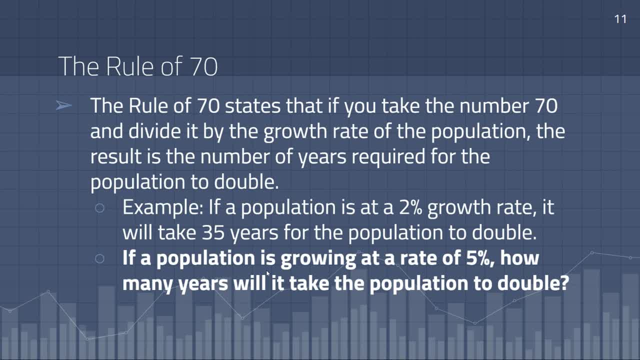 a population at a 2% growth rate could double. That's really crazy if you think about it. I'd like you to take a look at this practice question here. If a population is growing at a rate of 5%, how many years will it take the population to double? 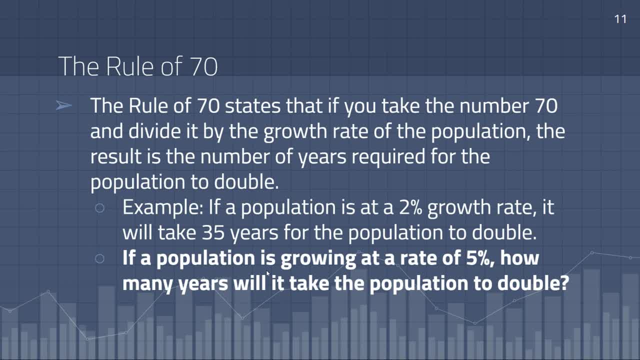 I'm going to pause the video here and try this question. Okay, so the answer to this question would have been 14 years. So if the population is growing at a rate of 5%, we would take 70, divided by that 5% growth rate, and we would get 14 years for that population to double. 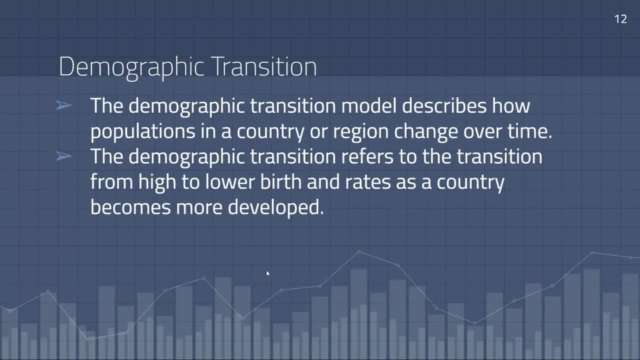 Okay, And finally, the last topic we discussed for this unit had to do with demographic transition. So remember that the demographic transition model describes how populations in a country or region change over time, And so the demographic transition refers to the transition from high to lower birth rates as a country becomes more developed, So as a country, 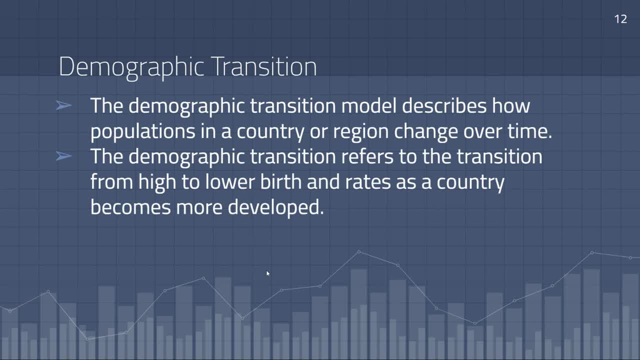 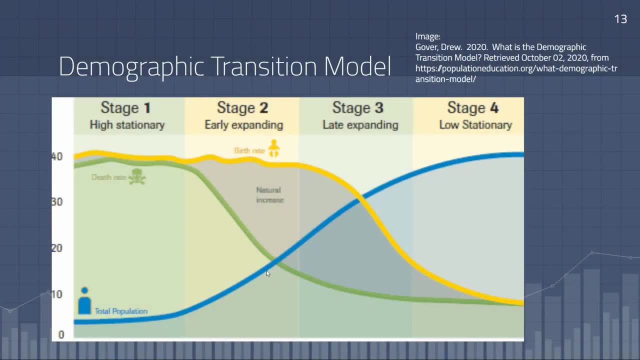 we're going to have more population, And so the demographic transition model describes how populations in a country or region change. over time, becomes more developed, we see some characteristic changes that start happening within the population, And there are four stages: to demographic transition or to the demographic 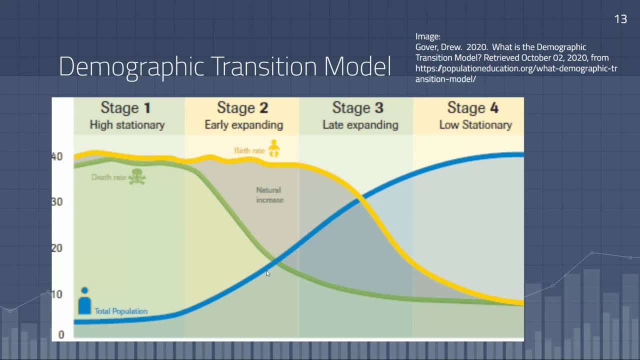 transition model. We can see the first stage represented here on this diagram And overall in this stage we have very high birth rates and high death rates, And so what we see is low population growth. There's not a whole lot of population growth happening If we look at 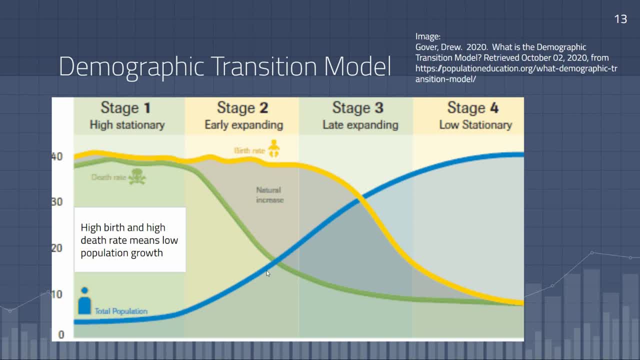 the blue line. that represents the total population. it's fairly stagnant in stage one. Moving into stage two, we start seeing some changes taking place. A country starts developing when it enters this stage two demographic transition model, So there's often a decrease in the death rate as the 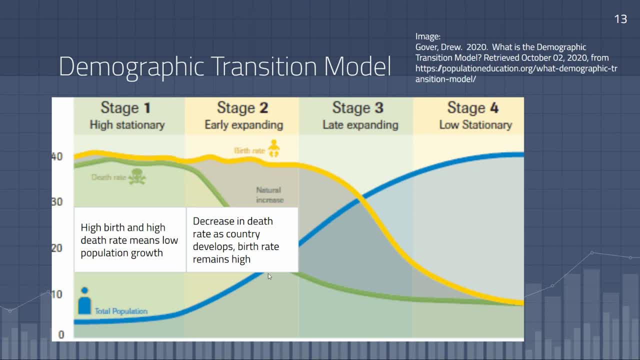 country's population increases And so we can see some changes taking place, So we can see some starts to develop. At this point, the birth rate still typically remains fairly high in that stage two of the model. So we have a decrease in the death rate, birth rate remains high. and what? 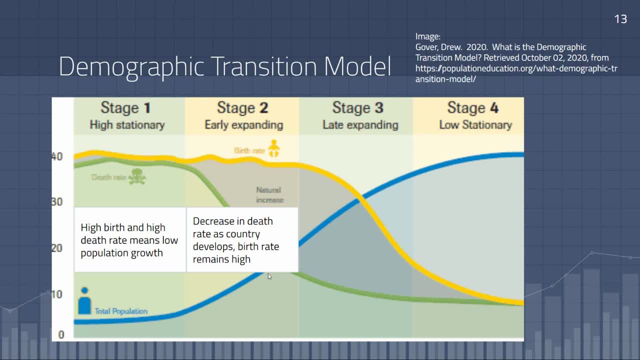 we're seeing here is a growing population, And then a country moves on to stage three in the model, And so during stage three we see low death rates, and we can see that represented by the green line here, And we also see that at this point the birth rates do begin to decline. And so here we